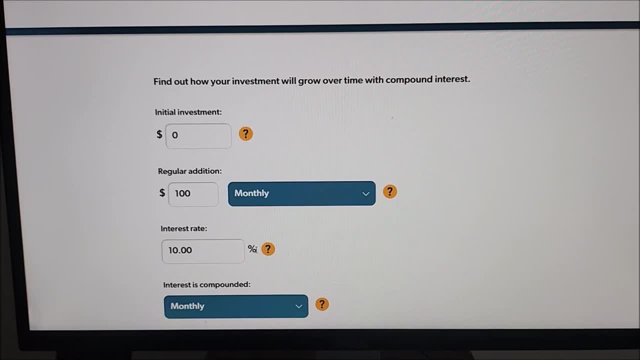 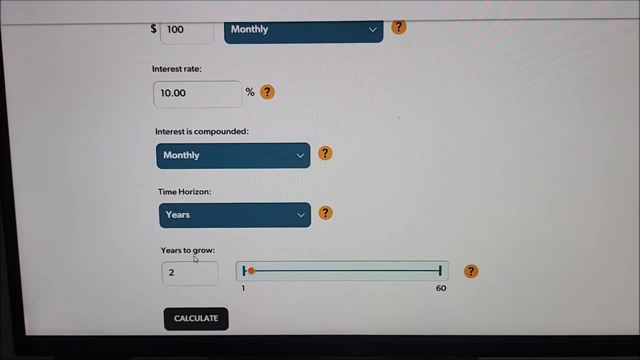 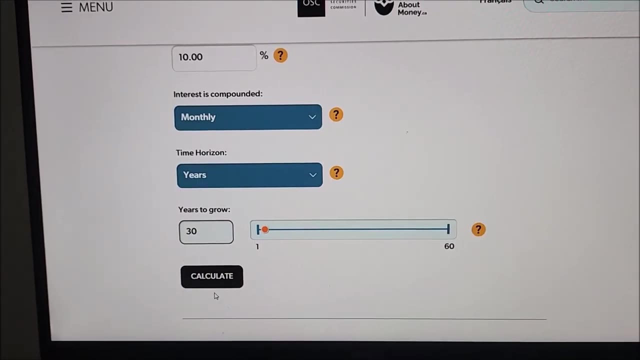 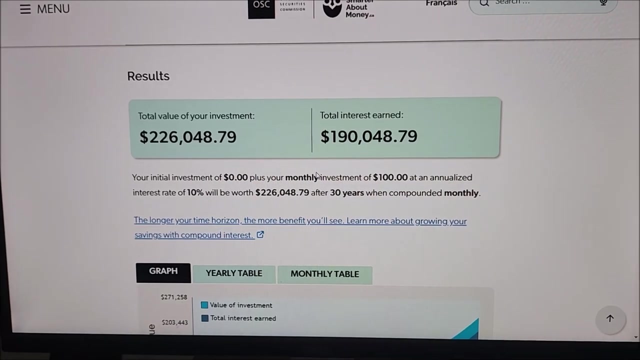 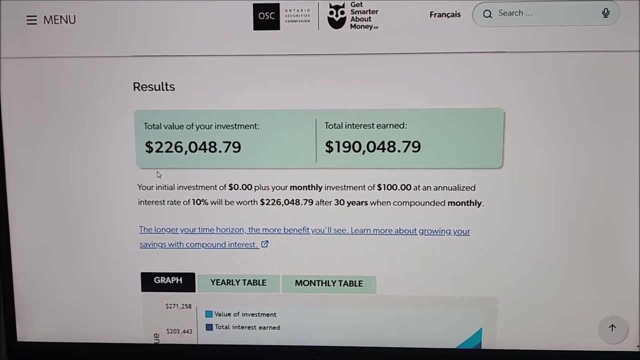 And I'm going to assume that the investments are going to be funds that are based on the S&P 500.. So I'll make sure I'll set this at 30 years And then I'll do a calculation. So let's say it's $190,000 of earned interest and the total value of the investment to be $226,000.. So let's say I change this to 40 years, The total investment of earned interest over the lifetime is over half a million dollars. So let's change the scenario. So let's say the initial investment is $100,000. And I'm not going to contribute anything. And let's say, same interest rate, but instead of, Instead of doing it for 20 to 40 years, I'm going to do it for, let's say, 10 years, Because let's say it took 20 years to save up $100,000. 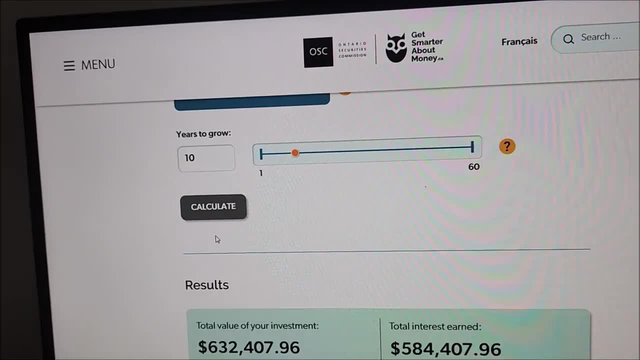 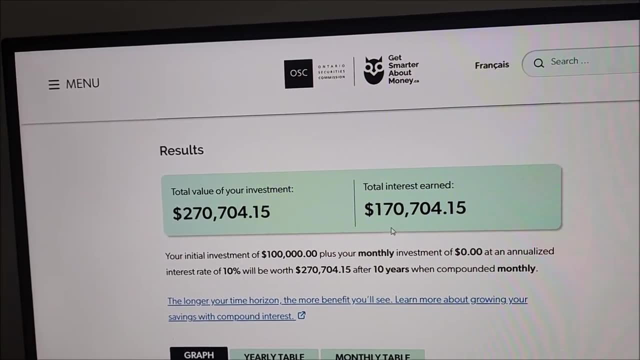 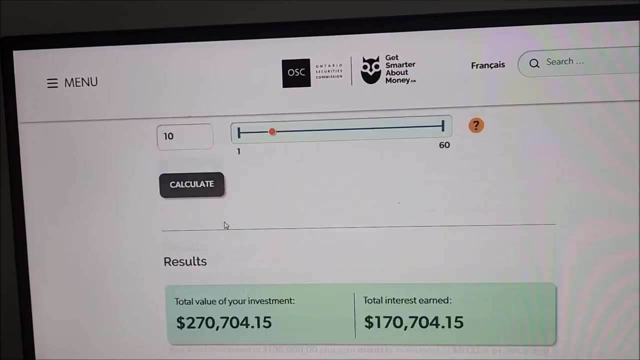 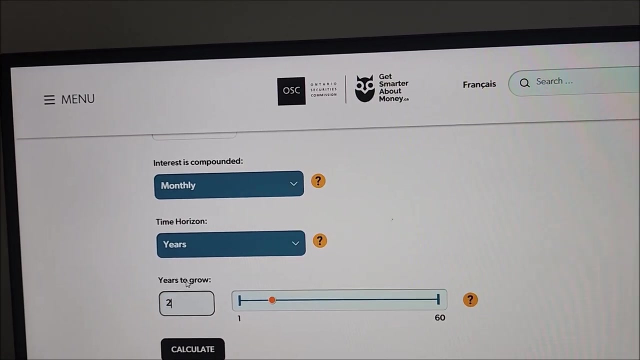 So let me just add $0 on this And the new calculation comes out to about $170,000 of earned interest And the total investment is $270,000.. So let's say I change this to 20 years. So similar scenario. 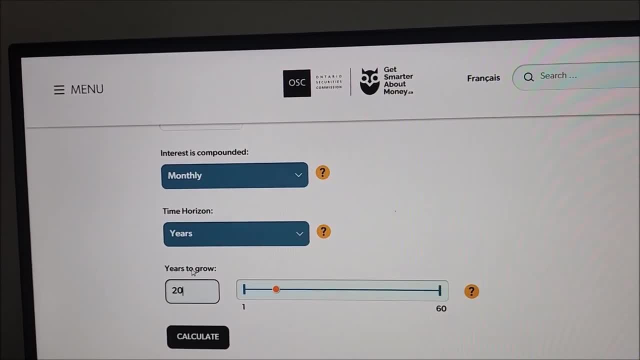 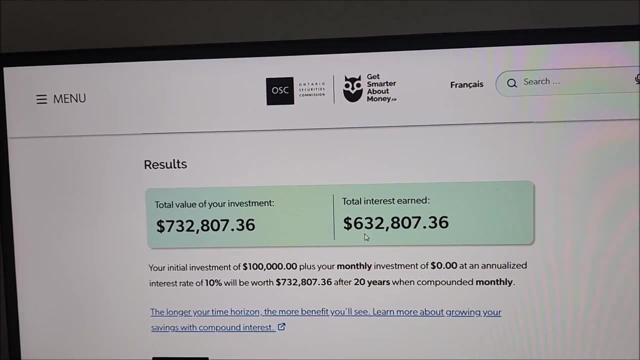 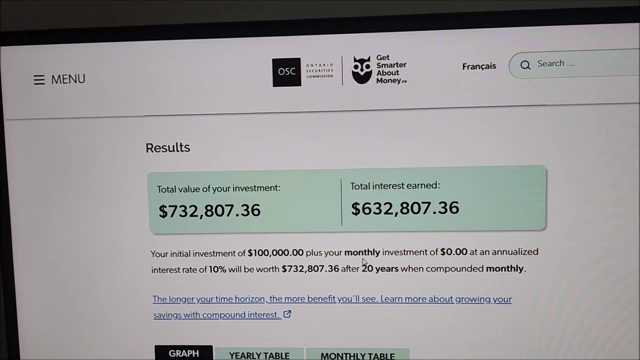 So you wait 20 years to save $100,000. And then now you invest for 20 years, So just a little bit over half a million dollars. So you can see how What a powerful time is. So you see how much the difference between 30 years of investing and 40 years of investing was. 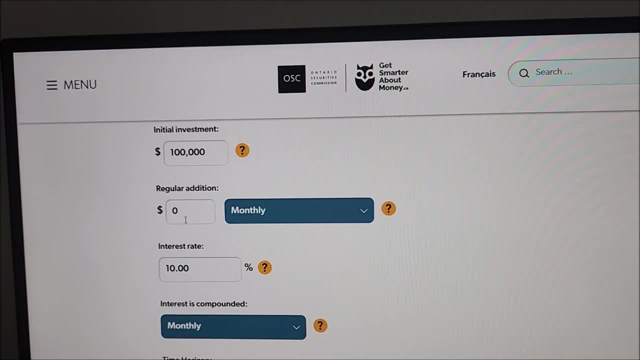 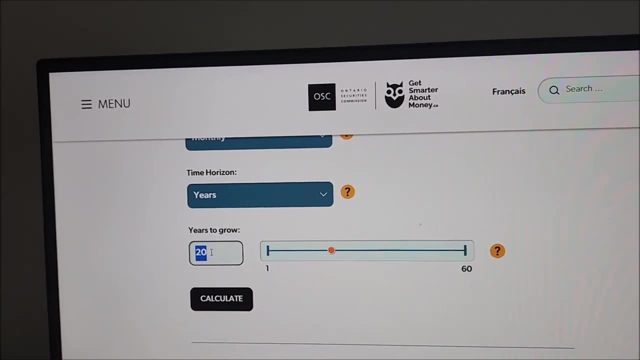 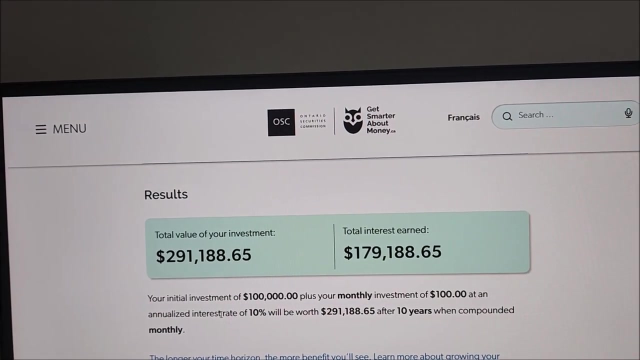 Now let's see if I change this to You save $100,000.. And now you add $100 a month, So it'll do this for, say, 10 years. So it didn't increase that much originally, So it was like $179. 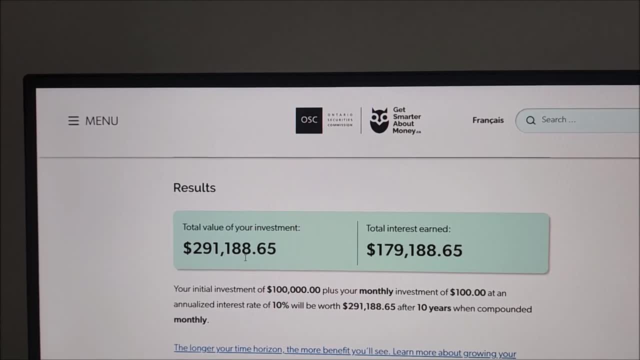 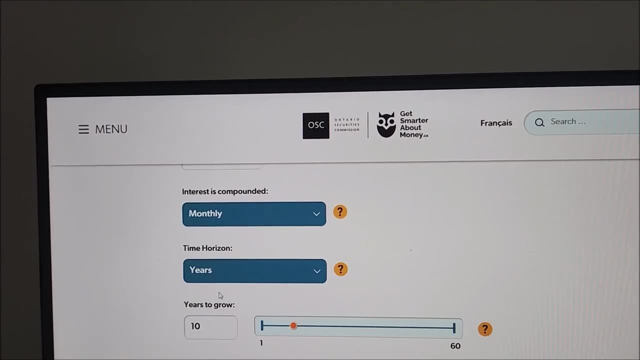 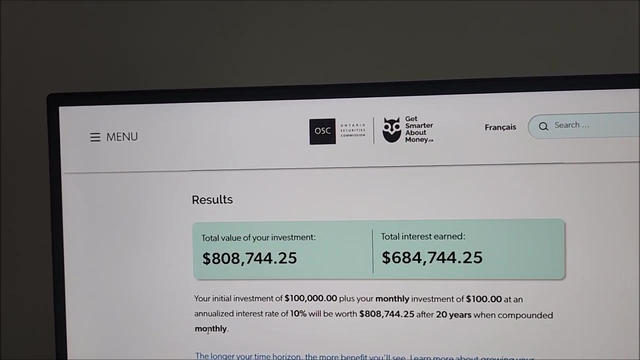 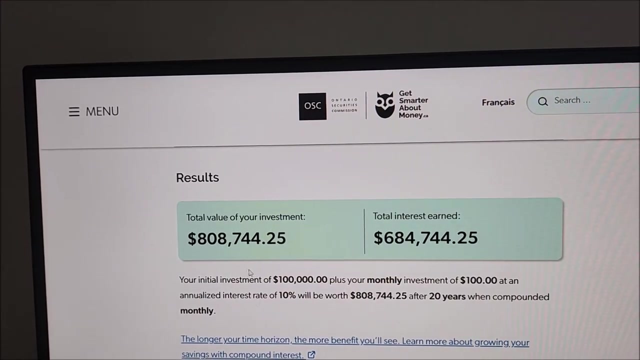 $179,000 of earned income And $291,000 of the investment. Now let's say I do this for 20 years, So it's just over half a million dollars. So $680,000 of earned interest With a total portfolio value of $808,000. 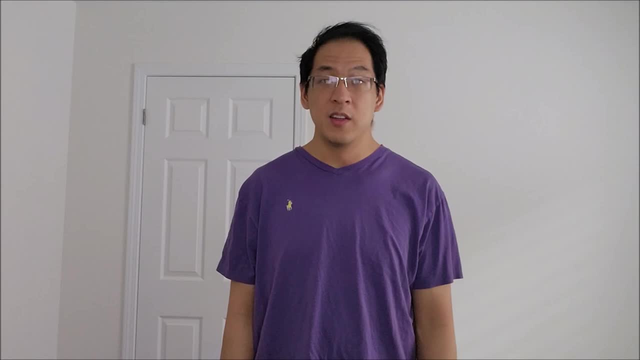 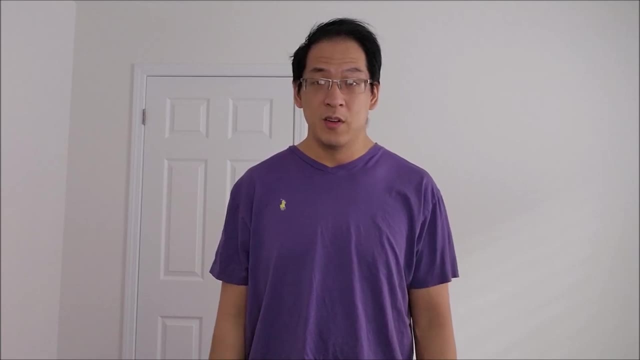 So I know the calculation is not accurate And it doesn't factor in taxes And it doesn't factor in the ups and downs in the share prices, Or if the S&P 500 goes down Or the S&P 500 goes up a lot. But I'm just basing this on a calculator, using 10% as an average rate of return, Because that's what a lot of people say. the S&P 500 goes up by, And I found that the first scenario seems to be a lot less stressful.